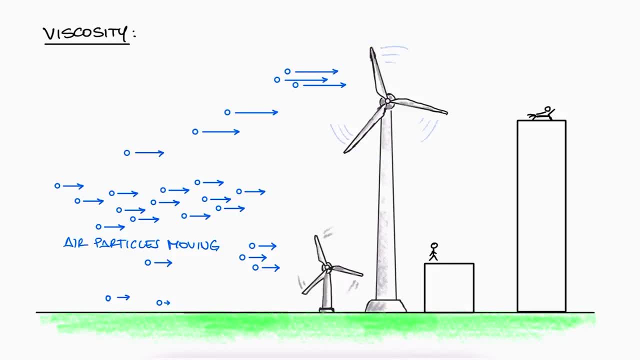 as it's reasonably possible, And it works both ways. The lower or closer you are to the surface where the fluid is flowing over, the slower it travels, So much so that, exactly on the surface, the speed of the fluid is exactly zero. 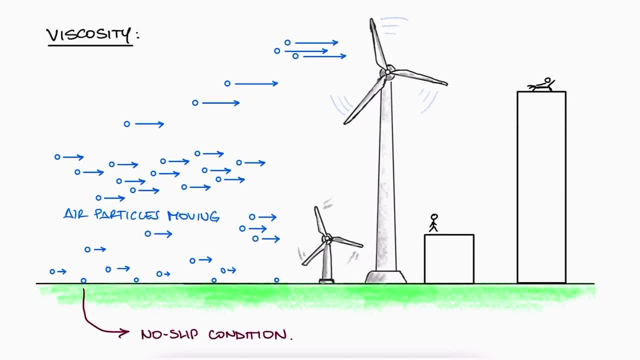 This is what's known as the no-slip condition. In general, a fluid that is in contact with a surface will have the velocity of that surface, whether that is zero or not. For example, if a fluid is trapped between two horizontal surfaces with a distance h. 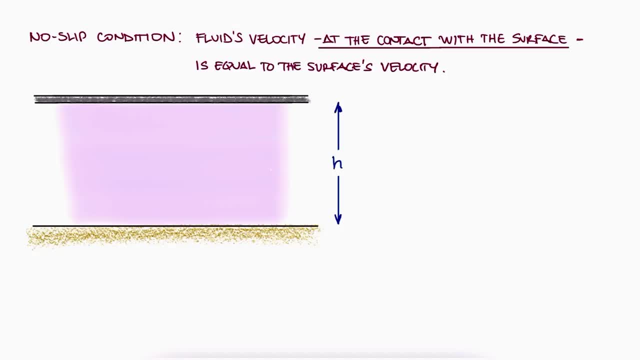 between each other, where the bottom surface is static and the top surface is moving with a velocity v. From the no-slip condition we know that the fluid particles at the very bottom are not moving and that the fluid particles at the top are moving with the same velocity v of 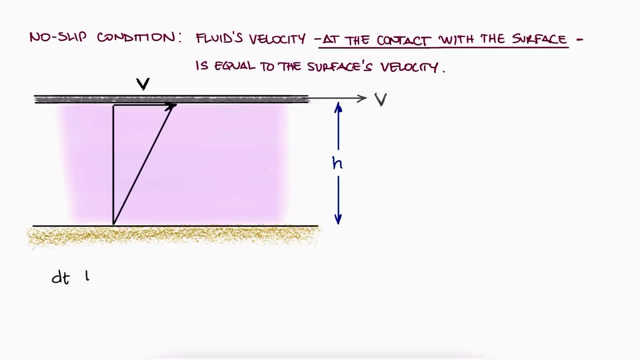 the top surface. After a small time, dt, the top plate will have moved dt times its velocity and we can call this dx That, or we can say that dx over dt is the velocity of the plate From the triangle that we see here. we can state that the tangent of the bottom angle 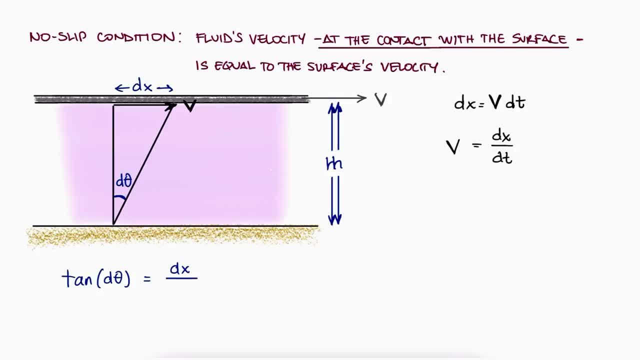 equal to the opposite side dx over the adjacent side h. Since this angle d theta is very small and if you remember from calc that the limit of tangent of x when x approaches zero is just x, then we can write this as d theta. 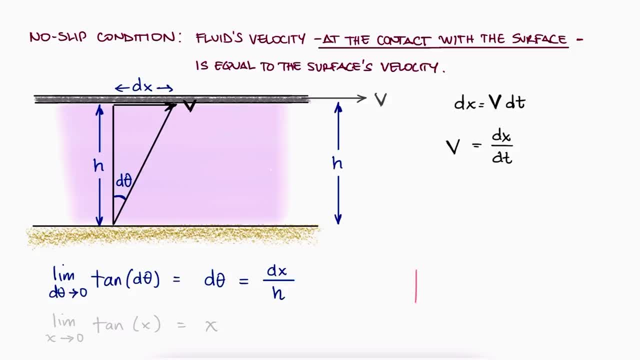 equals dx over h. From your mechanics of materials course, you probably remember a similar derivation. The small angle change is what we then defined as shear strain. in that case we used gamma. If we now divide both sides by dt, the left hand side is what we can therefore define. 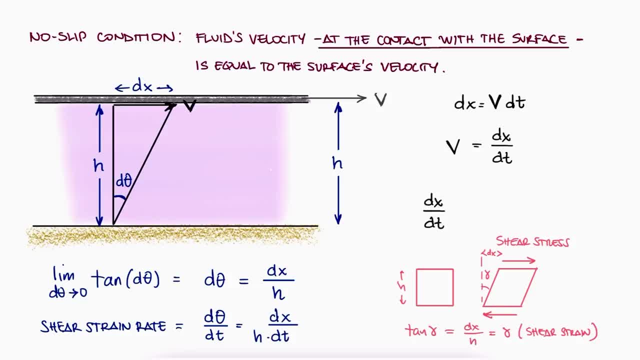 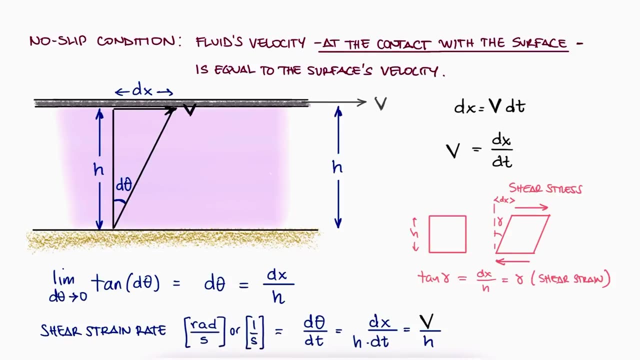 as the shear strain rate, and we see that the right hand side is the velocity v over h. The units of the shear strain rate are therefore radians over second or just one over second. Now we are not only interested in finding the shear strain rate at the top, where the 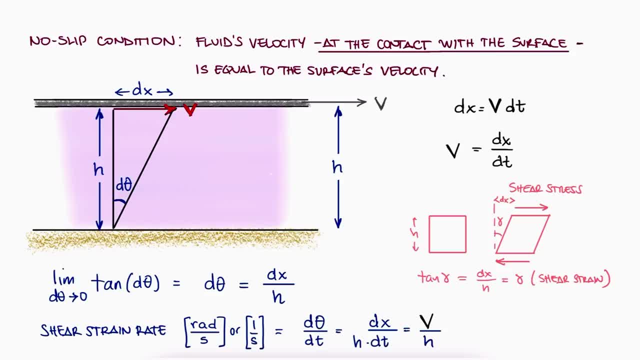 top plate is located fluid at any vertical location, dy as the velocity du. we know that v over h is proportional to du over dy. Now the connection between the shear stress- that term that we mentioned in our definition of a fluid- and the shear strain rate is very similar to what the relationship between 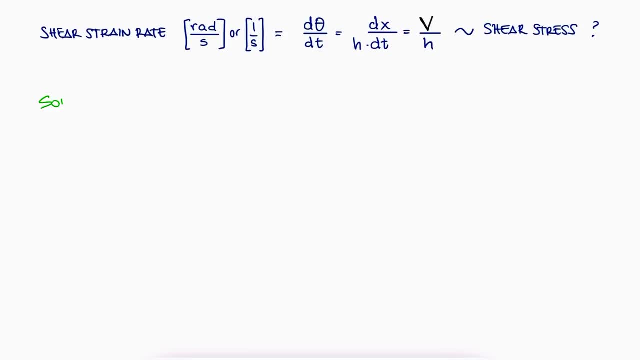 shear stress and strain is in solid mechanics. In that case we define that shear stress over shear strain is the property of the material that we call shear modulus or modulus of rigidity g. Of course, this linear relationship between the two is only true as long as the material is being 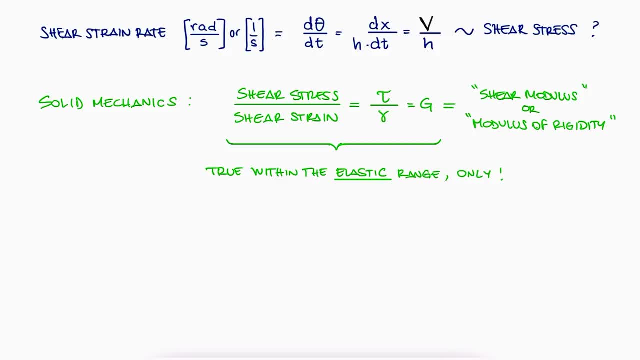 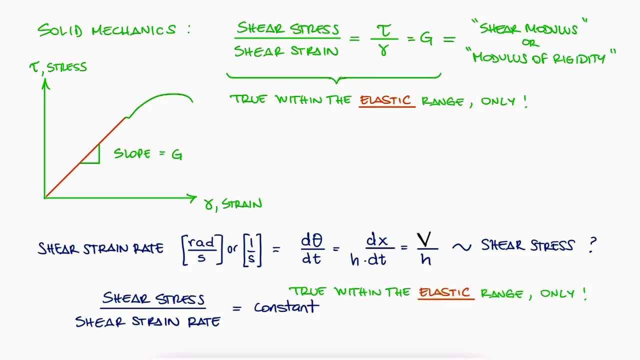 deformed elastically, not plastically. It is only true as long as we are looking at the linear deformation in a stress-strain diagram. Very similarly, here, the relationship between the shear stress and the shear strain rate will be linear as long as. 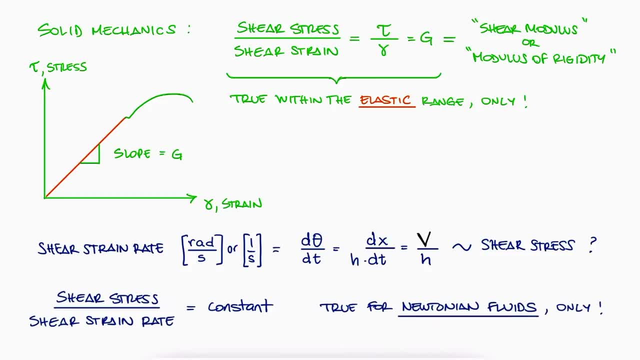 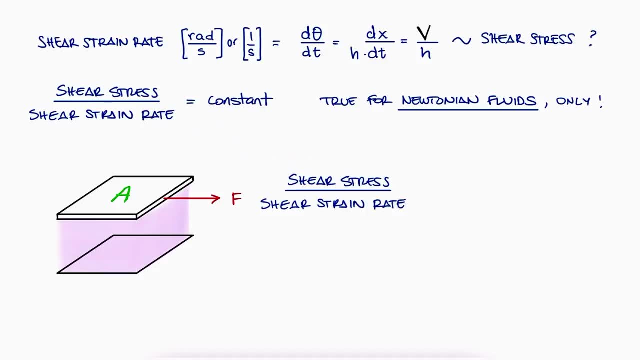 our fluid is what is called a Newtonian fluid. If we're pulling the top plate that has an area with a force, then the shear stress can be calculated as tau, equal to F over a, And just like in a solid material that is being elastically deformed. 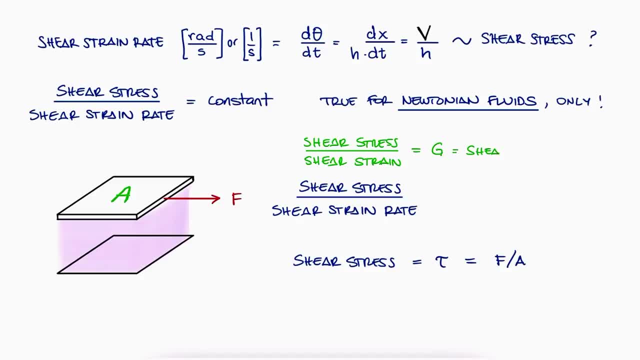 where the shear stress over the shear strain is a constant, called the shear modulus- here in fluids, but specifically to Newtonian fluids only- the shear stress over the shear strain rate is also a a constant that we will call viscosity. Now this viscosity is specifically the dynamic 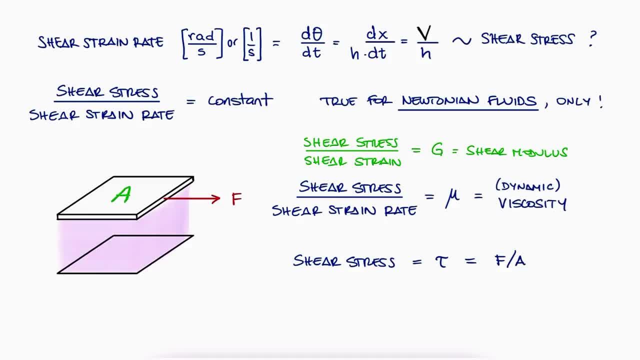 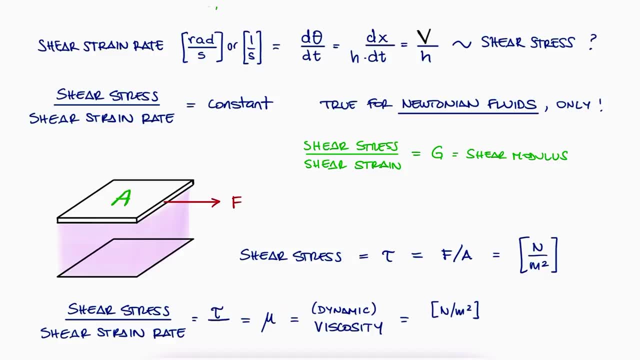 viscosity and we use the Greek letter mu as its variable. The units for dynamic viscosity in metric can be found by substituting newtons per meter squared for tau, one over second for the shear strain rate and rearranging to either pascal second or substituting newton. 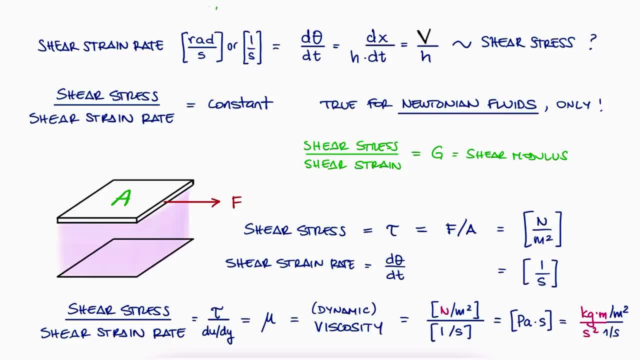 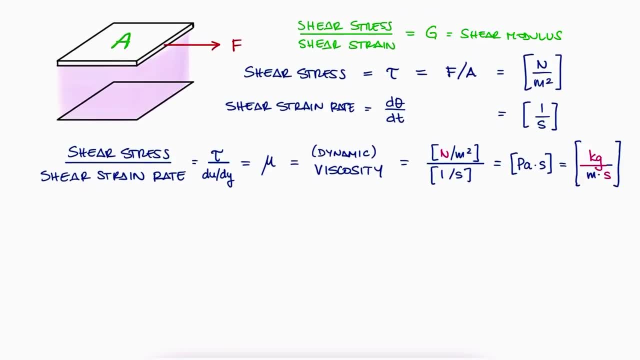 by kilograms meter over second, squared to write the units as kilograms over meter second. Going back to our analogy, just like we can plot the elastic portion of the stress-strain relationship between some metals, for example aluminum, a titanium alloy and steel meaning. 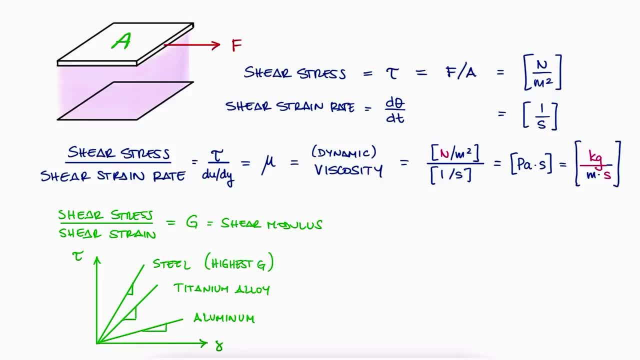 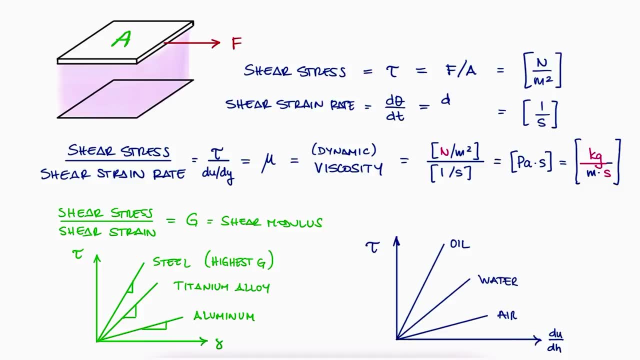 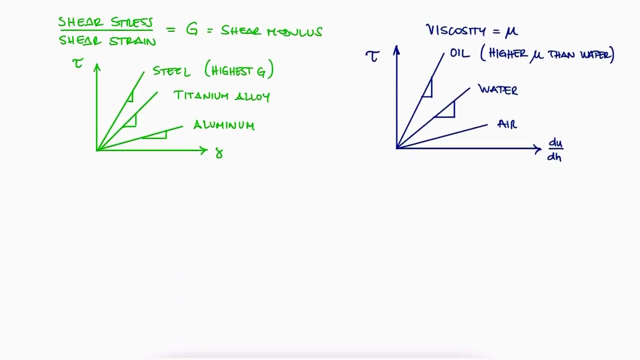 that the steel has a higher shear modulus and is therefore stiffer than aluminum. we could plot air, water and oil on a shear stress versus strain rate diagram to say that oil is more viscous Now, since we will be using the density of the fluid for many of our calculations, like 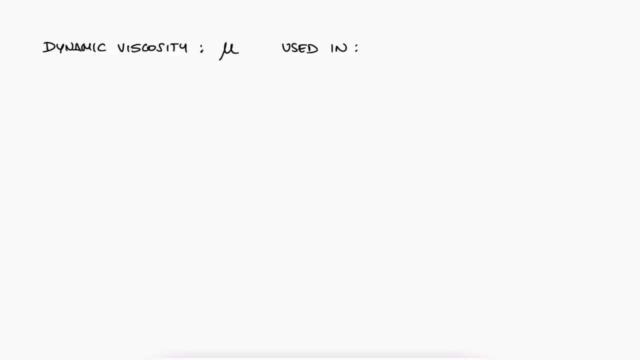 it was stated a few minutes ago, and the density is usually next to our dynamic viscosity, mu. we can also define what the kinematic viscosity is with the letter nu as the dynamic viscosity over the density of the fluid. By substituting the units of each, we see that the kinematic 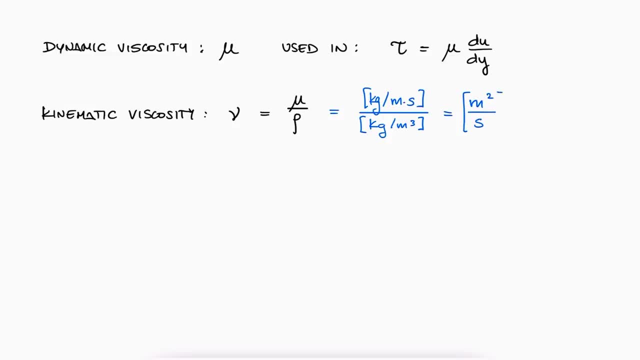 viscosity nu has units of meter squared over. second, An easy way to remember this is that kinematic, which means motion, should be similar to velocity, which has units of meters per second. In this case, there's just an extra meter on top. 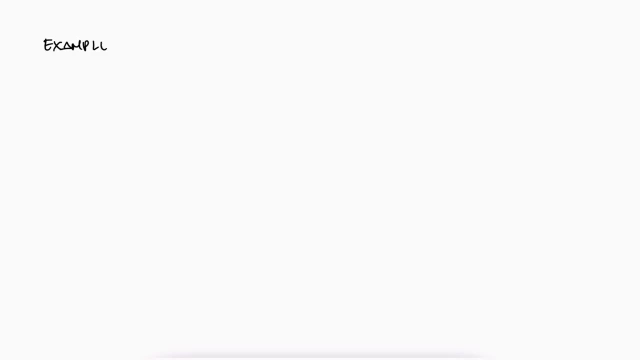 Let's look at a simple example where we make use of what we've learned today and if you want to check out more examples on this topic, some of them using English units too, any other of the lectures of this fluid mechanics course, like Bernoulli's equation or head? 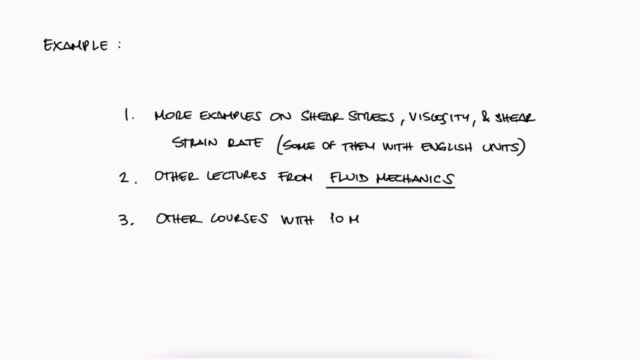 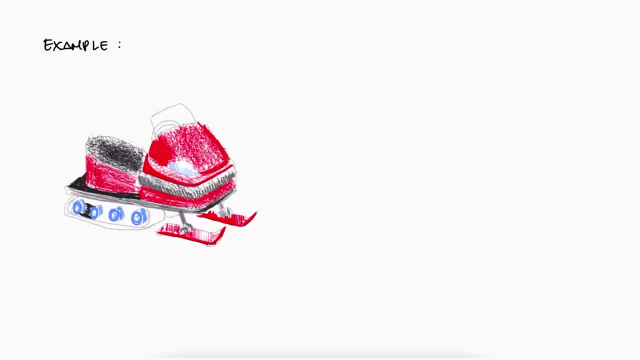 loss calculations or even playlists of other engineering courses. make sure to check out the links in the description below. Let's say there's a snowmobile that reached an area that is covered in ice instead of snow. Between the sleds and the ice there's a very thin film of water, 14 microns in thickness. 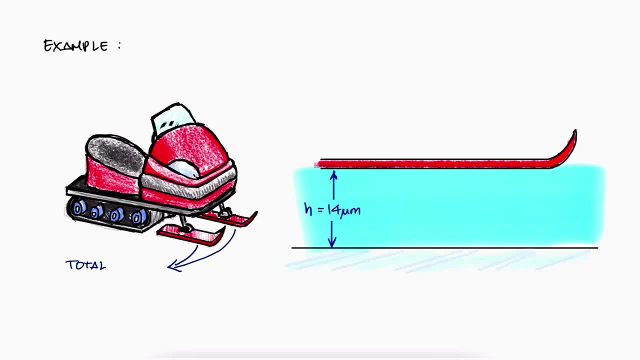 and the total contact area between the sleds and the water is 960 squared centimeters. What is the thrust force that the snowmobile should generate to maintain a constant speed of 40 kilometers per hour? A simplified schematic of the sleds over the ice, over a thin film of water, would show a rectangular. 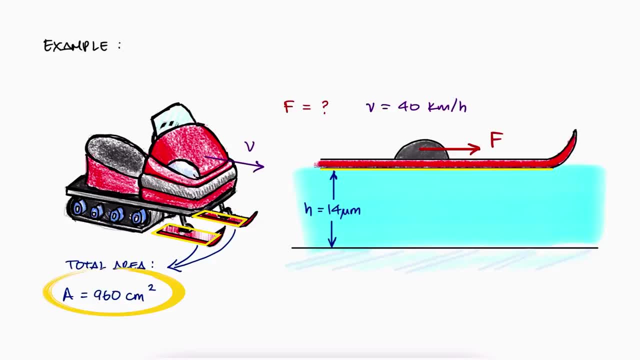 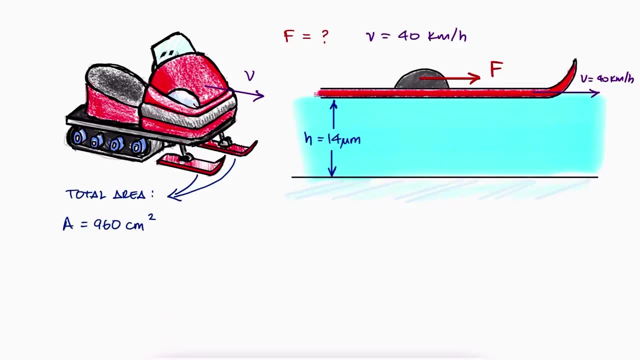 plate to the sleds of area 960 squared centimeters, 14 microns above the static's ice surface, with water between them. The shearing stress would therefore be the viscosity of the water times. the shearing strain rate du dy, Since v over h is the same as du dy or the slope. 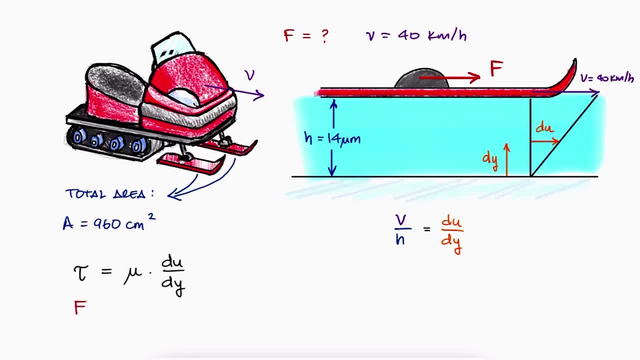 of the diagonal and the shearing stress. tau can be written as the force that is being applied to the snowmobile over the area. we can solve for the force and calculate its value if we find the viscosity of the water first. To do that, and since we know that,